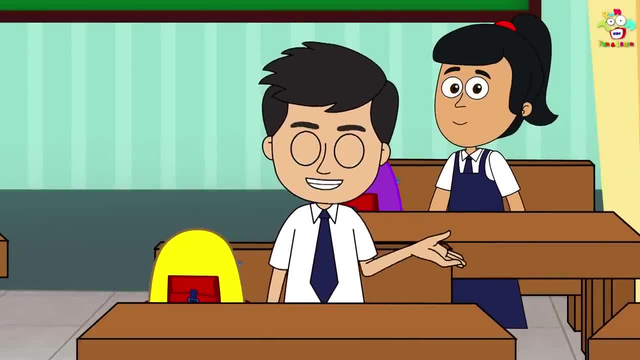 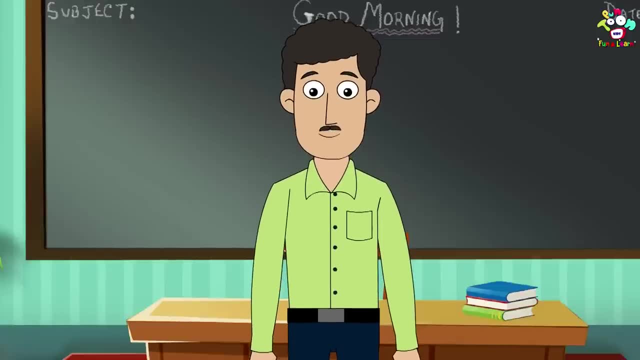 Sir Krishna Janmashtami is going on. There was a Dahi Handi festival in our society, So we couldn't do our homework. No problem, kids, Don't worry about your homework. Tell us what happened in Dahi Handi festival. 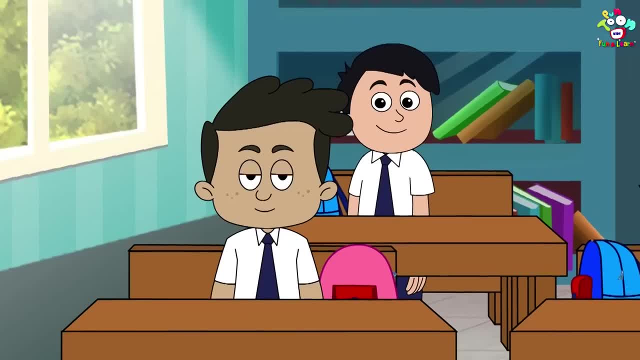 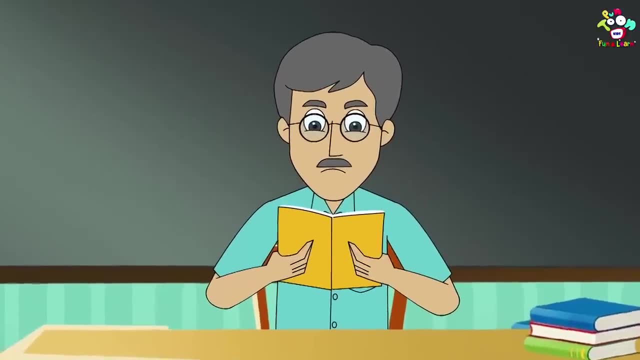 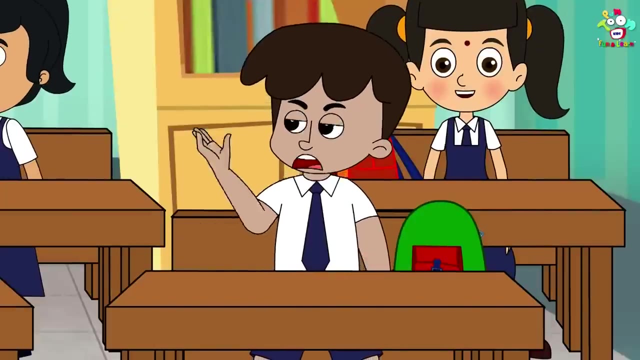 Today we will talk about Dahi Handi in class. Now, if a teacher says this, then why would the children worry? But there was a teacher in Gattu Chinky's school during whose classes children used to feel tensed. Gattu, give me some water. 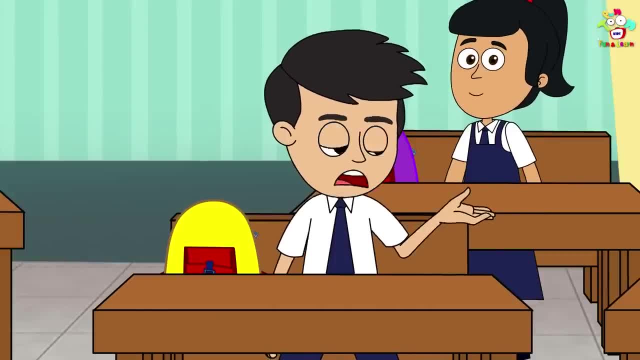 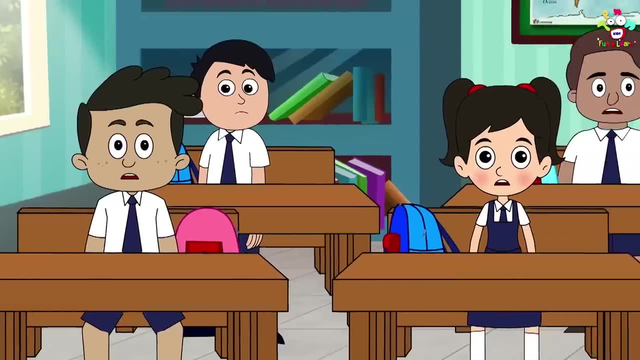 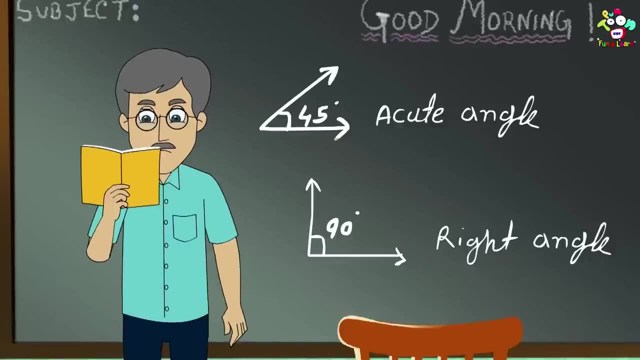 No, no, I'll also need water. Mishra sir must be coming. Sadakant Mishra was no less than Hitler for the children During his period, the whole class would be quiet before he arrived. Absolutely pin drop silence. Mishra sir used to teach maths. 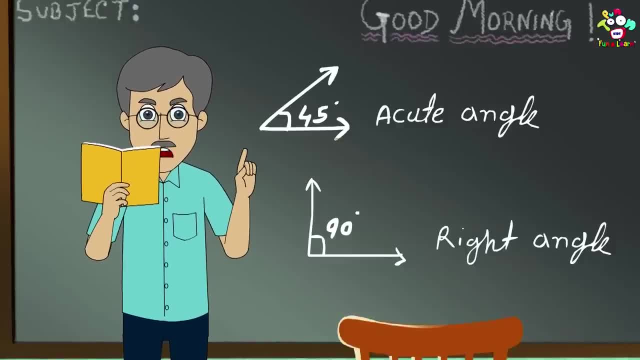 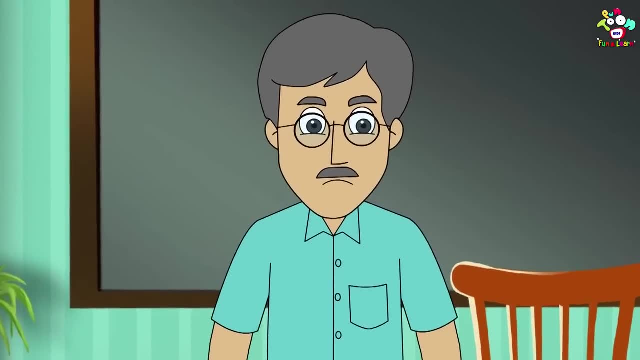 Along with that. he was a serious type of man. He himself followed the discipline and wanted the children to follow the discipline too. Mishra sir came to the class, turned his eyes on the whole class and started solving maths problems after seeing the children sitting in discipline. 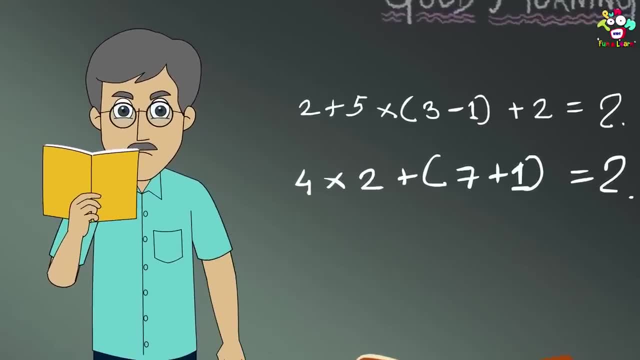 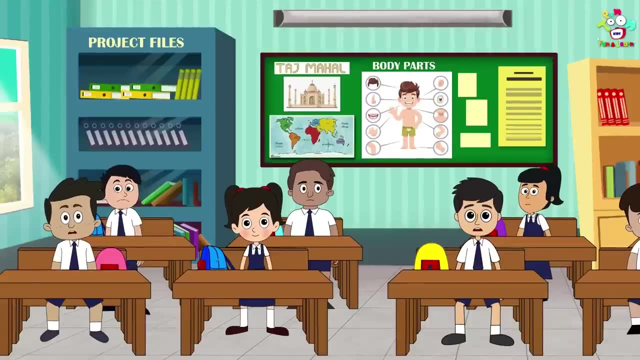 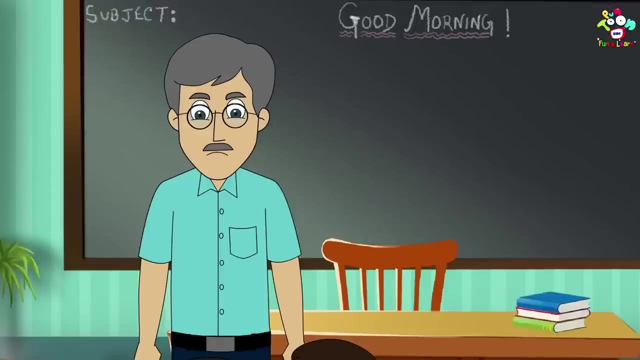 Mishra. sir's class was about to end when Chinky said, Sir, you gave us homework yesterday. You didn't check the homework. Hearing this, everyone's heart started beating faster and the whole class gave Chinky an angry gaze. Why are you staring at her? 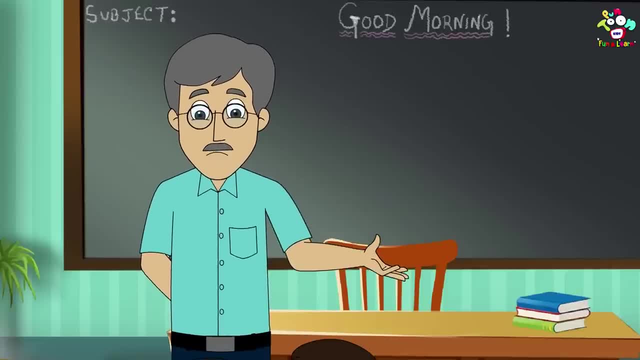 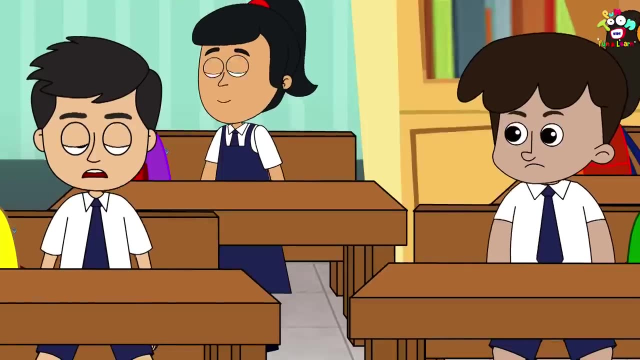 Except for Chinky. I want everyone's notebook on my table. Not a single, Not a single kid came forward. Mishra sir again looked at the kids. Gattu, say something, Say something, Gattu. Why don't you say? 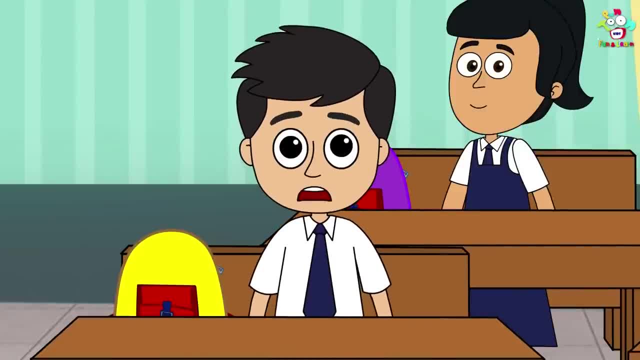 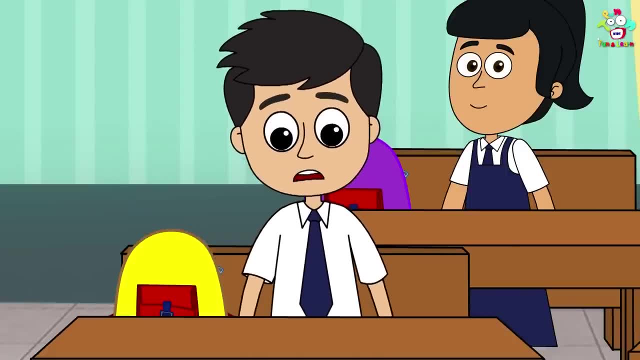 What's the matter, Gattu, Sir? Sir Krishna Janmashtami was going on, So there was a Dahi Handi festival in the society. So homework. Now imagine what Mishra sir would have done to the children after hearing this. 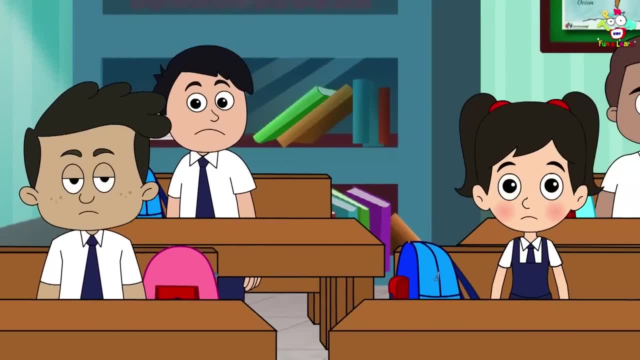 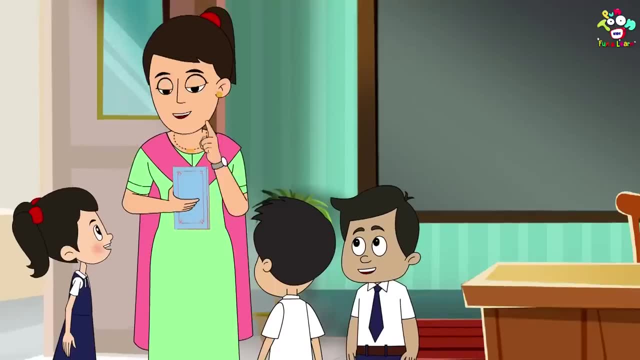 This was the reason why none of the children at home would listen to this. This was the reason why none of the children at home would listen to this. This was the reason why none of the children at home would listen to this. The children who attended this festival were always like Mishra sir at school. 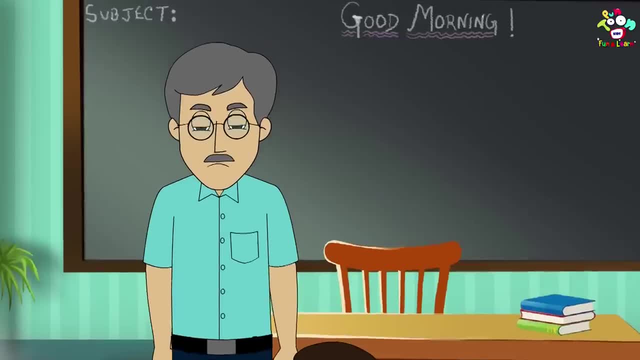 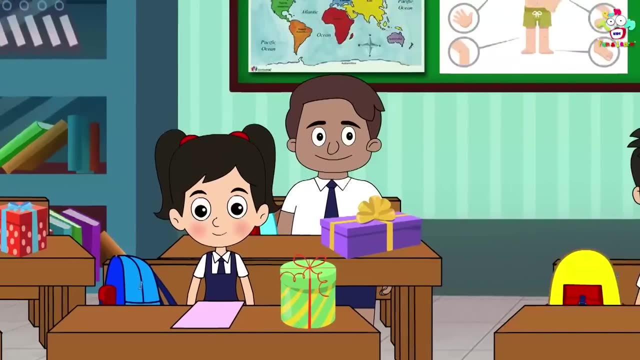 And always ran away from him. There was always a crowd of children behind the rest of the teachers, But Mishra sir, He always used to be alone. September 5th was Teachers' day. All the children brought a lot of gifts and greeting cards for their teachers. 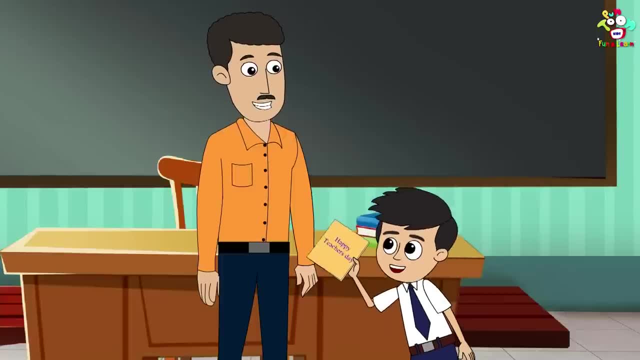 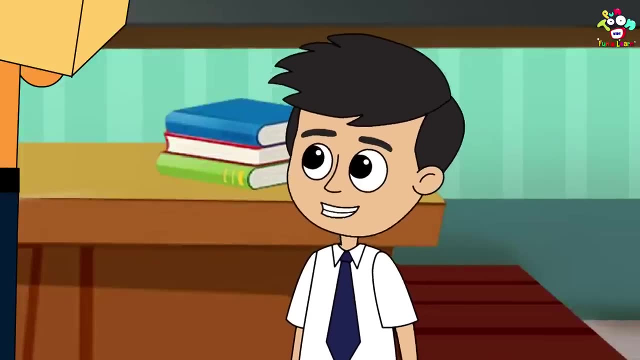 All the children brought a lot of gifts and greeting cards for their teachers. Happy Teachers' Day, sir. This is for you. Oh, Thank you very much, Gattu. Have you made this greeting card? It's very beautiful. Thank you, sir. 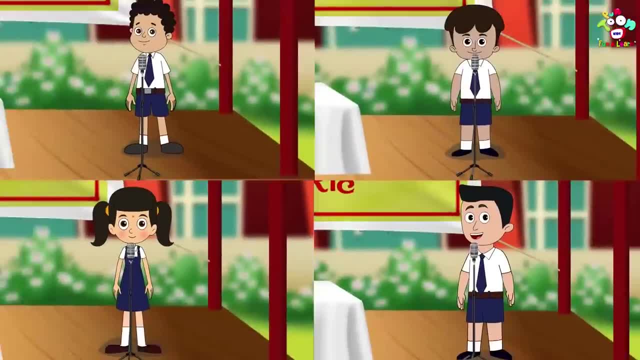 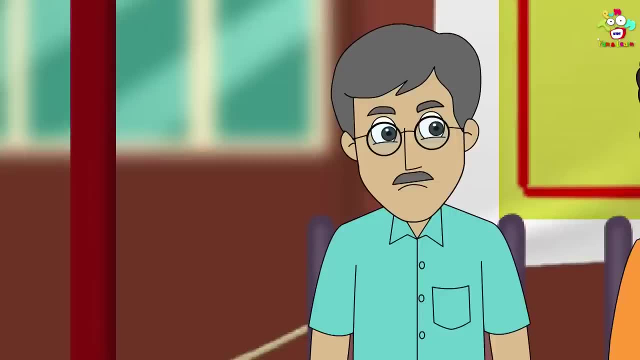 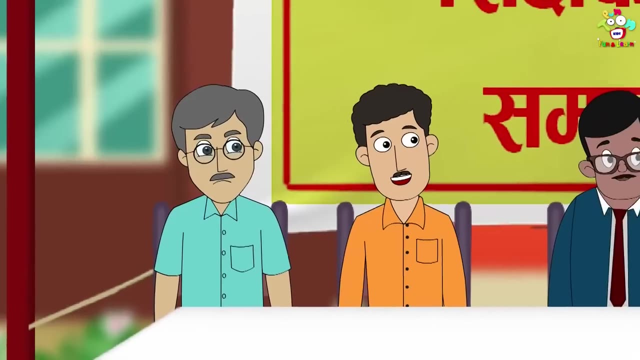 During the celebration of Teacher's Day at school, all the kids were talking sweetly about all the teachers And all the teachers were happy to hear their praise. But none of the children ever took the name of Mishra sir. Even no one wished Mishra sir or gave any greeting cards. 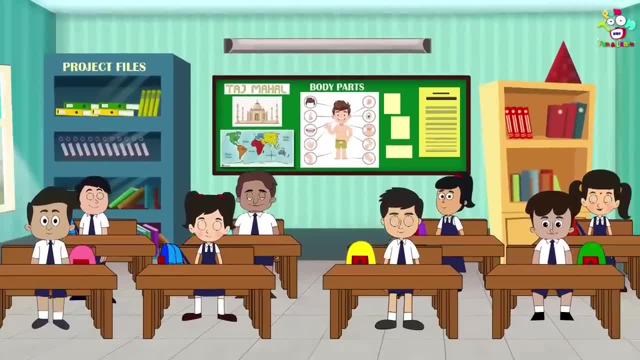 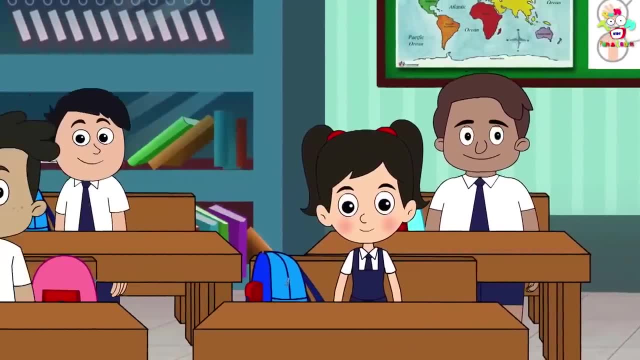 The children sat in the class and started studying. After a while, the maths period started. Everyone sat down and waited for Mishra sir. It was quite late Still Mishra sir did not come. Hey, he will not come today to take class. 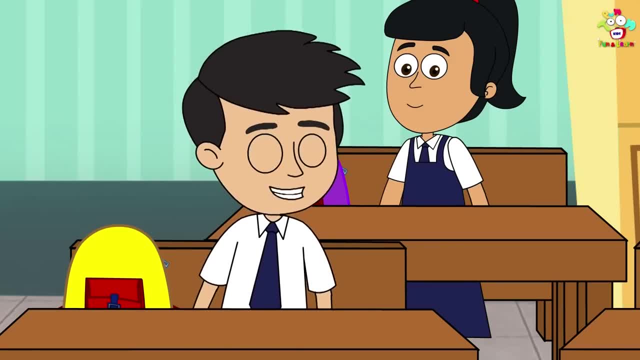 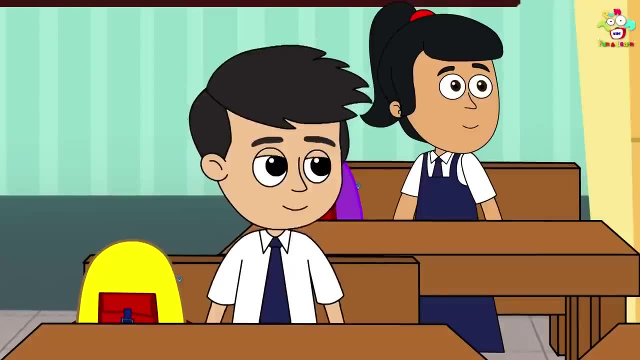 He has been unwell since morning Means no mathematics for today. That's when the peon came to the class and said: Children, Mishra sir is not well, We know. So there will be no maths class for today, right? 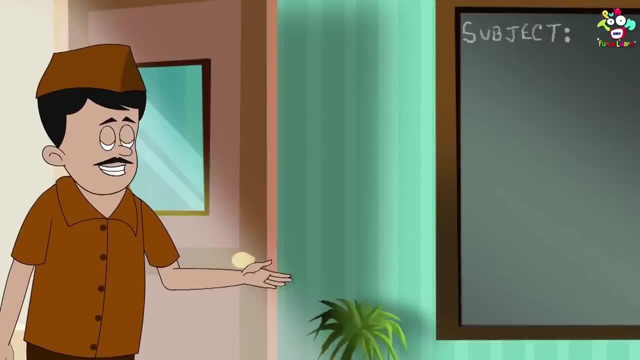 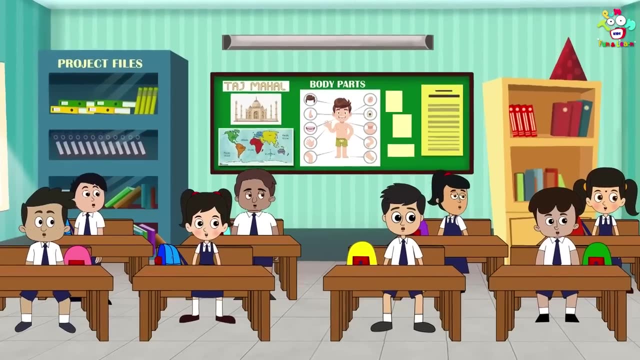 Oh, no, no, He is not well. He cannot even walk, So he won't be able to come to the class. You all have been invited to the teacher's room Today. he will be taking your class there. Hearing this, all the children were shocked. 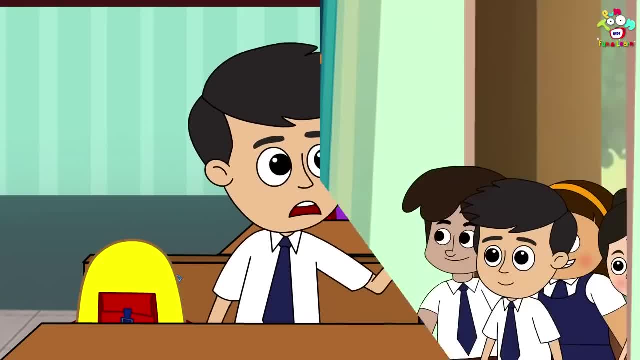 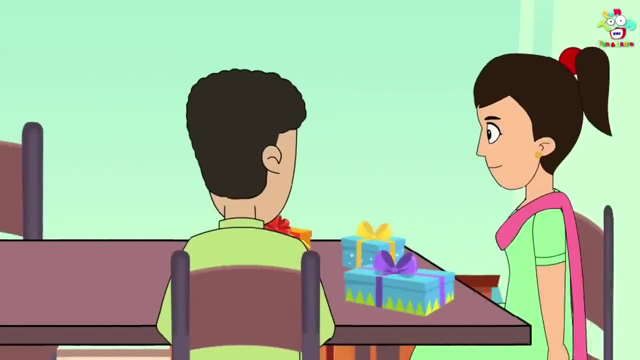 What is this? If he was sick, why did he come today? When the children reached teacher's room, they saw that there were a lot of gifts and greetings in front of all the teachers, But Mishra sir's table was completely empty. 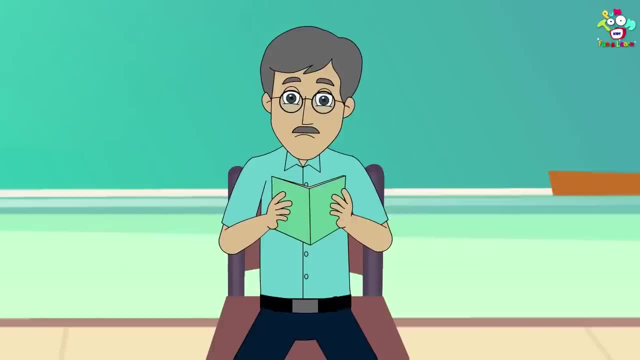 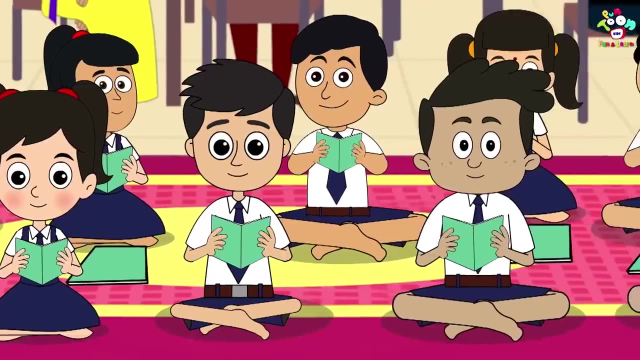 The children sat down and Mishra sir started speaking. Sorry kids, I am not well today. Come on Now open your books. The kids took out their books and the class started. Then the peon came and said something in the ears of Mishra sir. 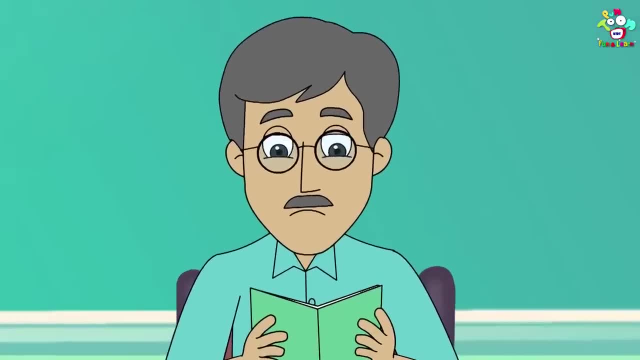 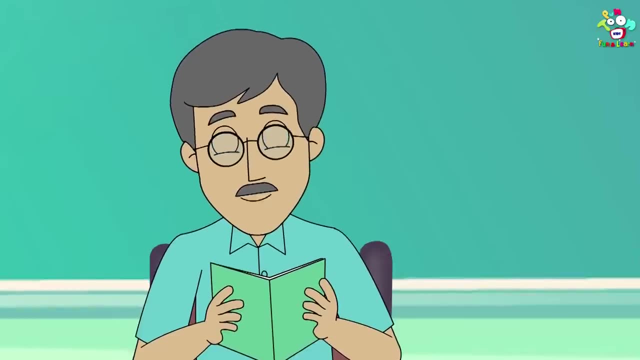 Not now Tell him to wait. Mishra, sir, kept taking the class. After a while the peon came and said: Sir, can I send him inside Five minutes more? The children did not understand what was happening. The class got over. 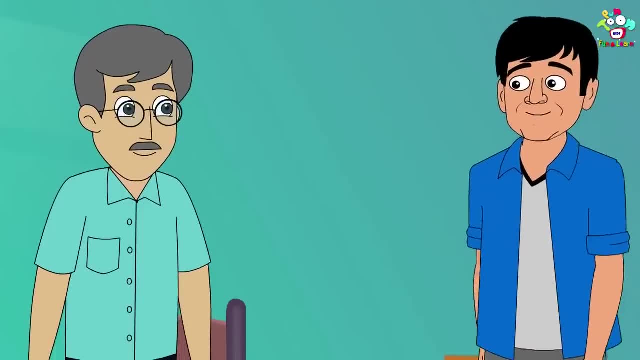 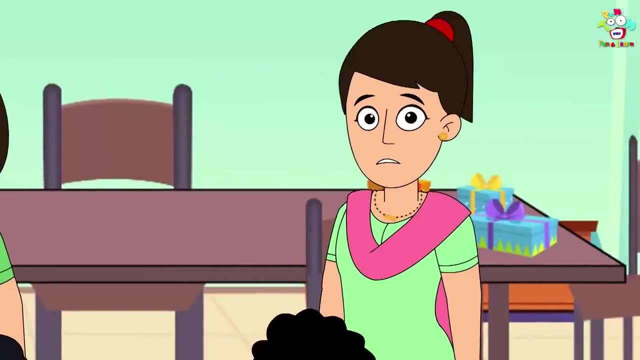 The children were shocked. They were about to leave. That's when a person came inside and touched Mishra sir's feet, Seeing which, along with the children, the entire teacher's staff also got shaken. It was Dheeraj Chopra, who won the gold medal in Olympics for India. 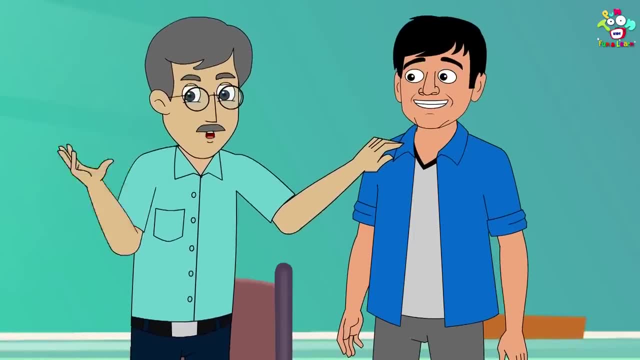 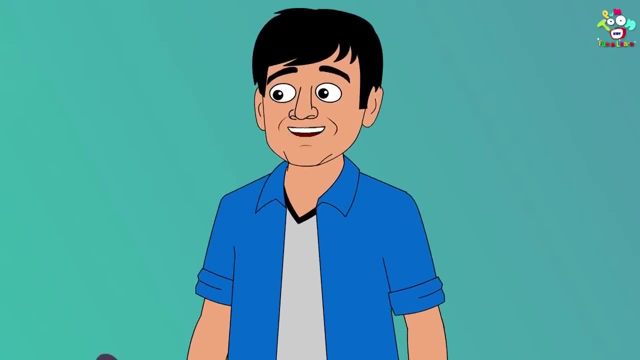 Oh, Dheeraj, come in Children. you go to the class, Please, sir. We also want to meet Dheeraj, sir, Why not, Sir, please, let me meet the kids. Okay, Dheeraj, Come sit here. 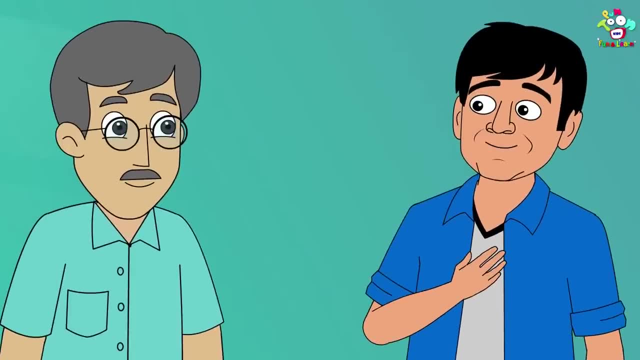 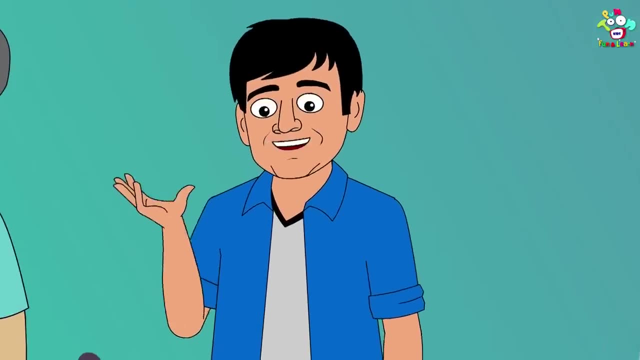 No, sir, I will always stand in front of you, Just like you used to keep me standing in the class. Remember, Children, you will be surprised to know that your Mishra sir has been my class teacher And whatever I have achieved today, 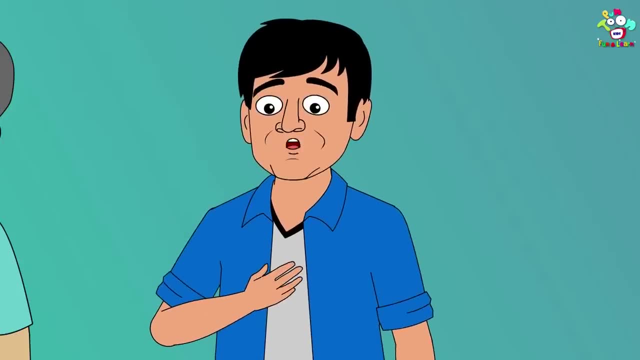 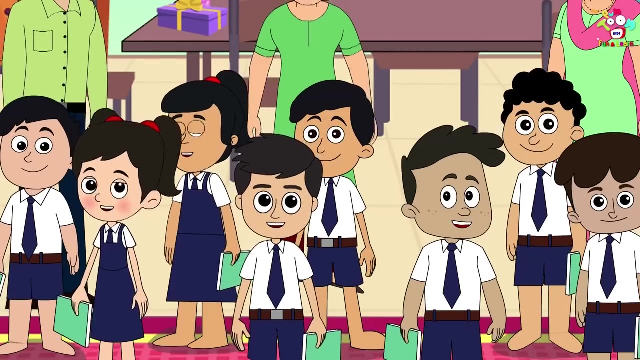 it's only because of him I was very weak in studies. I used to run away from school. Then he used to scold me a lot. He must have scolded you too, As soon as he came to know that I was interested in sports. 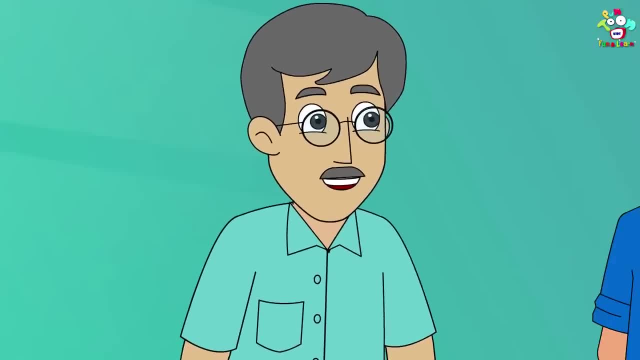 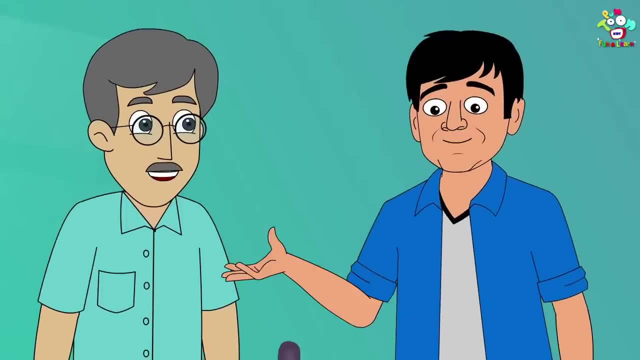 he started taking my practice on the ground for two hours after school. He was my first coach. He taught me discipline. That is why I could achieve all this in my life. Children, you must be thinking: why didn't I receive any gifts or greetings on Teacher's Day? 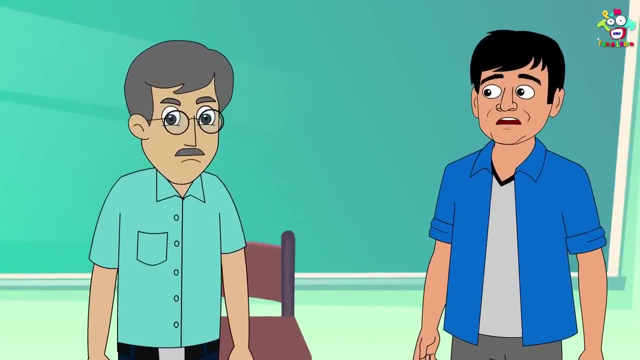 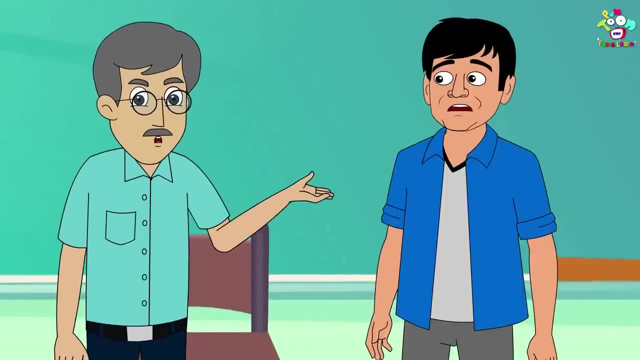 No one gave me anything because I am very strict. I cannot change it because it is my teaching pattern. But today, on the occasion of Teacher's Day, let me tell you it's not like I haven't received any gift. I did receive a gift, but a little late. 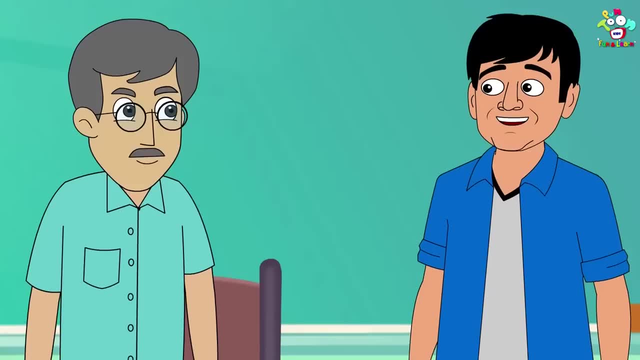 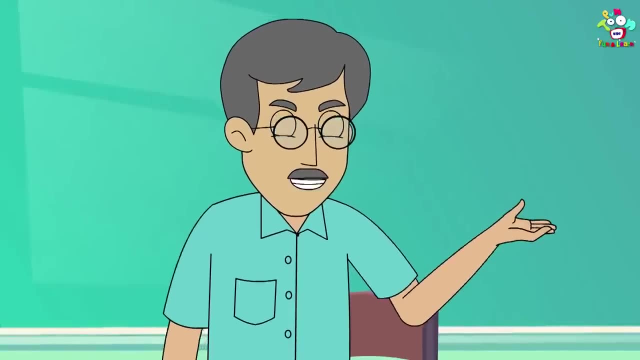 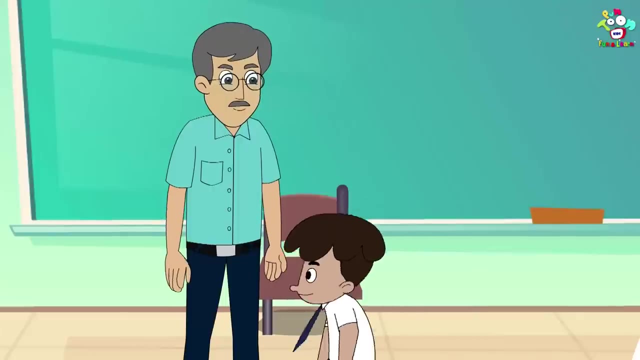 Look, Dheeraj has come as my gift. Do you know, Tomorrow any of you will come as my next gift? The success of my students, this is my biggest gift. Hearing this, all the children became emotional. They realized their misunderstanding. 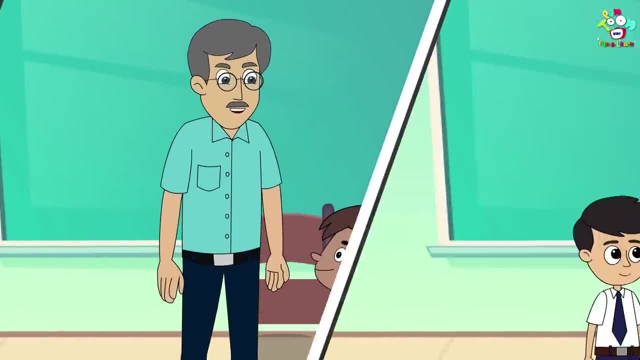 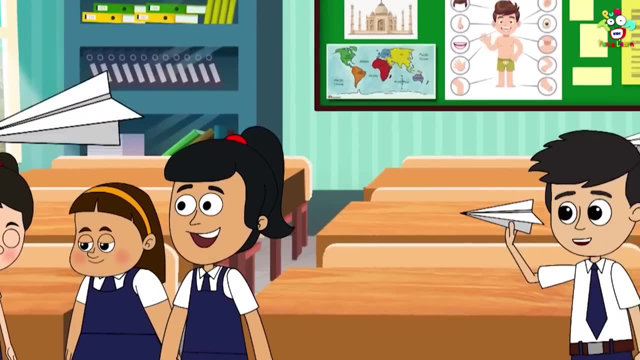 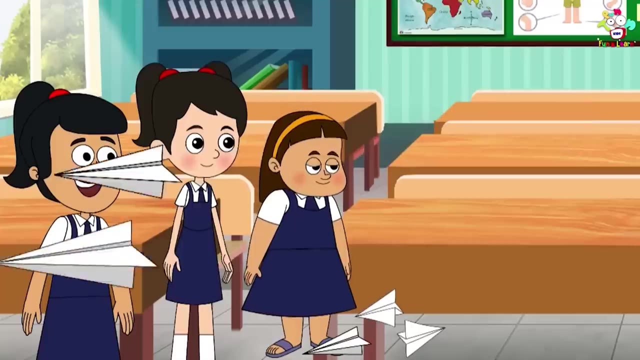 and they bowed down to Mishra sir and started seeking blessings from him. Gattu and Chinki were playing along with their friends in the classroom. Come on, boys, attack Girls. let's teach them a lesson. Pick the aeroplane and attack them. 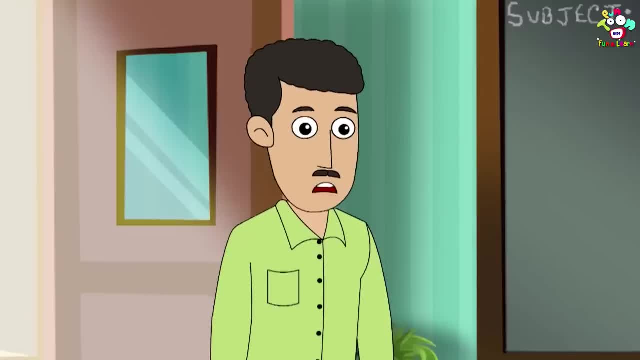 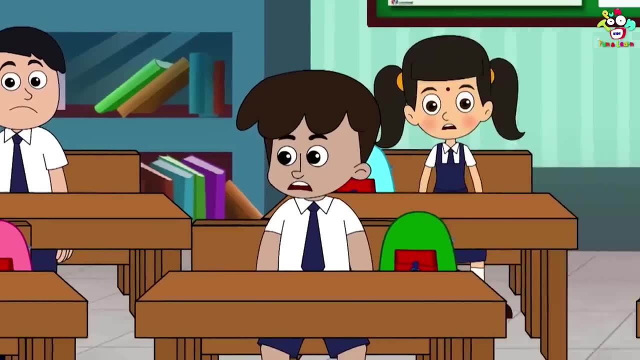 That's when Mishra sir enters the classroom. What is all this noise? Within two minutes, I want everyone to bring their homeworks and put it on the table. Hearing that everyone starts looking at each other because none of them have actually done the homework. 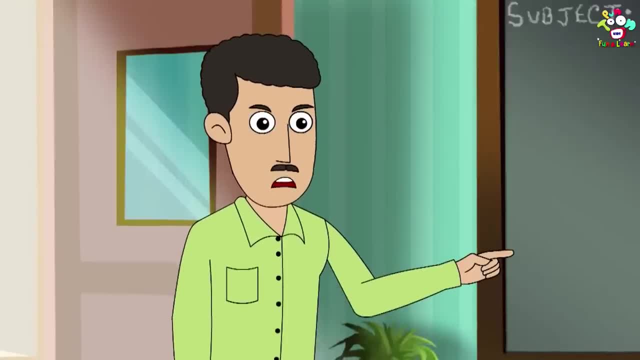 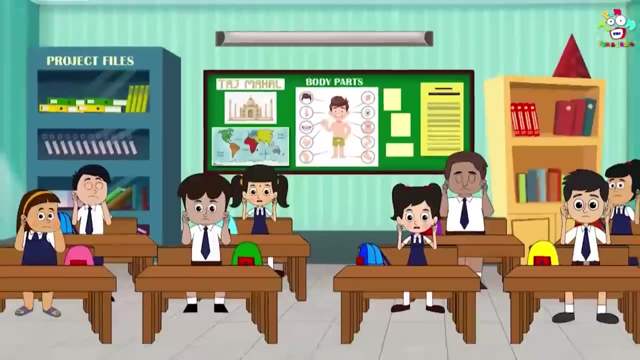 Nobody has done the homework. You all just know how to misbehave in the class. Now all of you get up and hold your ears. Come on, do it fast. The entire class stands holding their ears and that's when Piyul comes there with the circular. 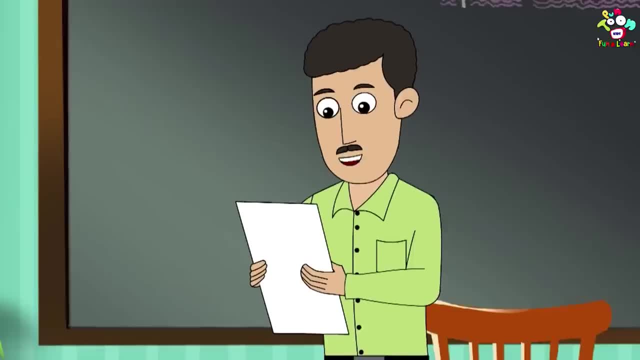 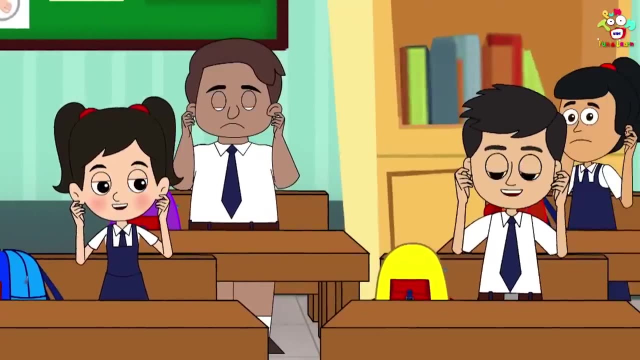 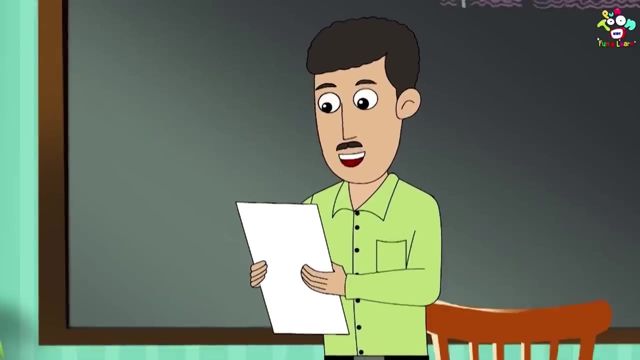 Teacher's day circular. sir, All the teachers are hereby informed that the teacher's day will be held in the respective classroom. All the students should prepare their own plan and offer greetings to their teachers Immediately after reading the instruction. all the teachers are requested to be in the meeting room. 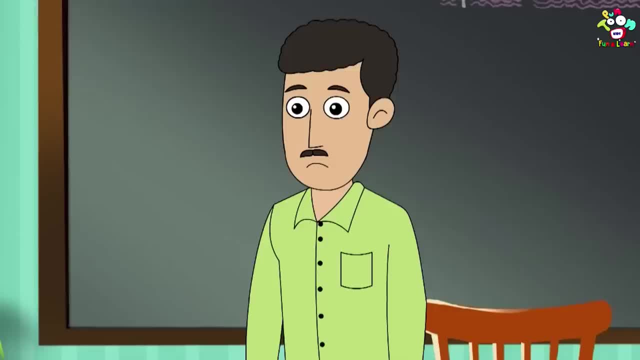 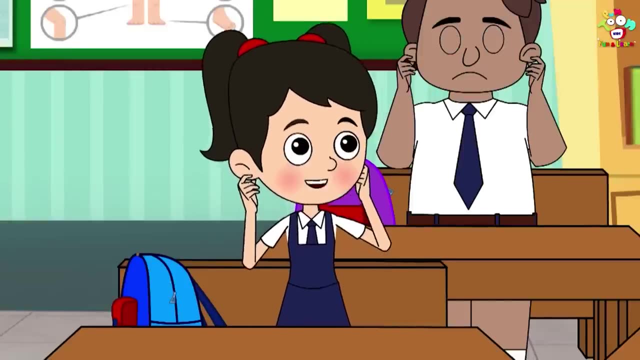 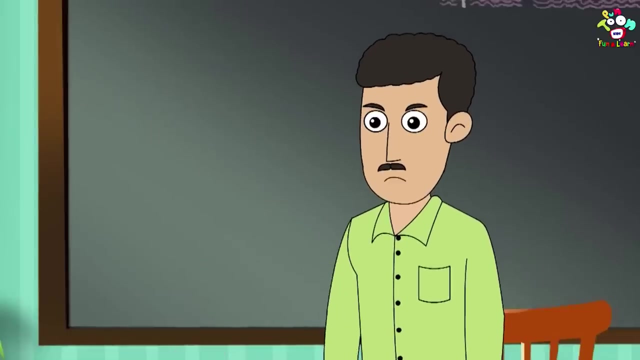 So, sir, can we sit now? Why do you want to sit, Sir? you need to go and meet principal and we need to do teacher's day, planning, Planning, or want to make noise once again? My punishment hasn't ended yet. Now I'm going to give you all double homework. 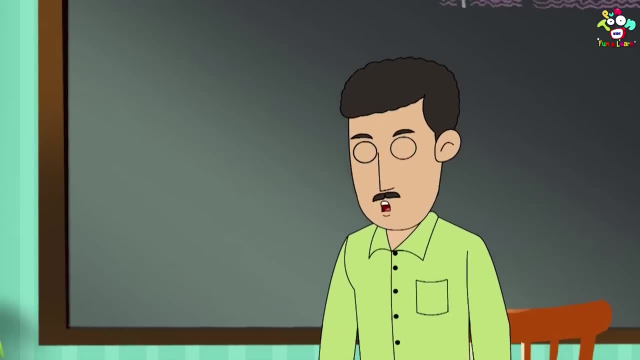 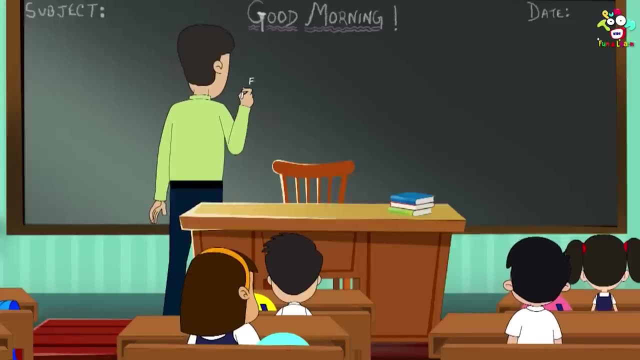 and if it's not finished by tomorrow, you all know what punishment I'll give. Sit and open your notebooks now. Kids sit and open their notebooks. Mishra sir writes a lot of homework for the kids and leave for the staff room. Oh friends, so much homework. 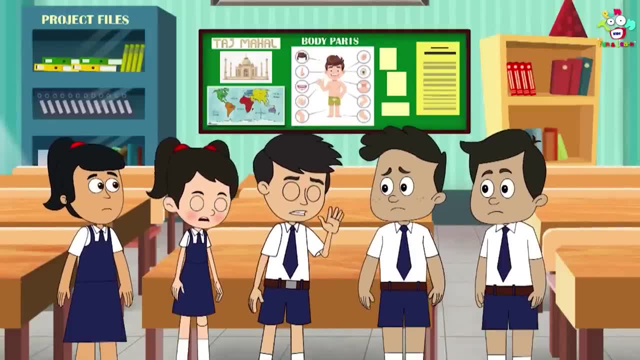 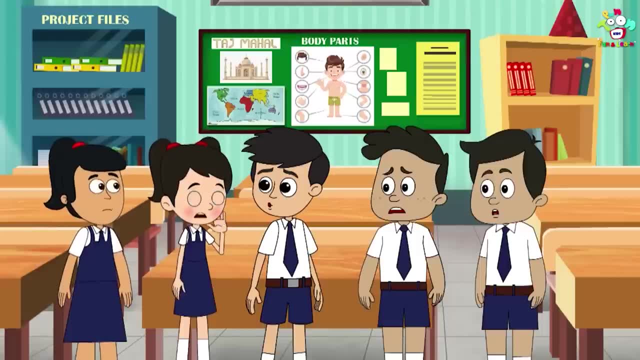 Even if we sit all night, we won't be able to complete it. Mishra sir is angry on us. That's why he gave so much homework. If we don't do it today, tomorrow he'll punish us. Now what to do? 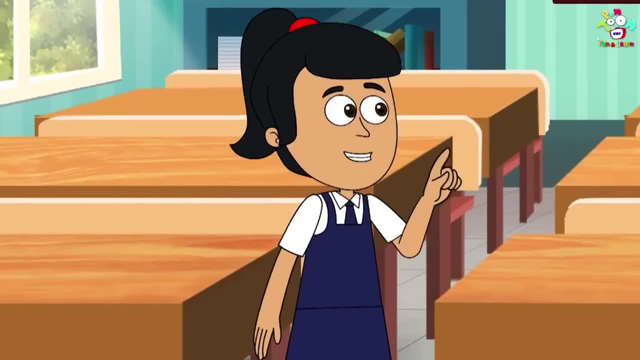 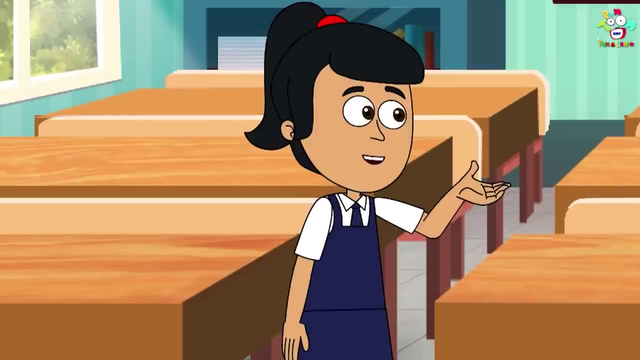 That's when Rani gets an idea. Tomorrow is anyway teacher's day. We have to do all the planning. If we take lot of gifts for Mishra, sir, he will be very happy And then he won't punish us. Brilliant idea. 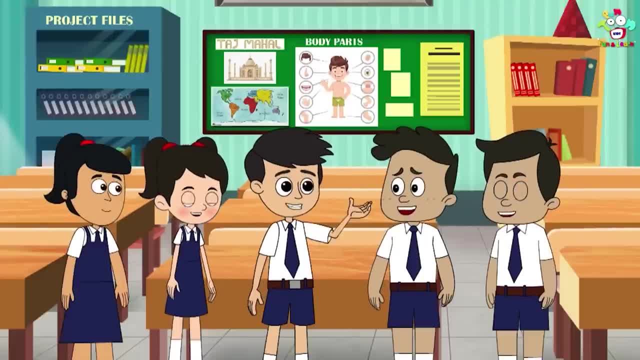 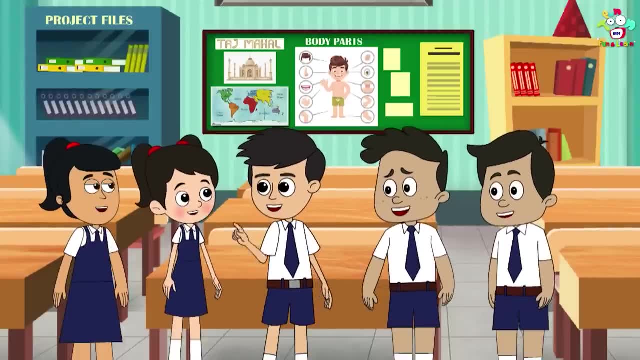 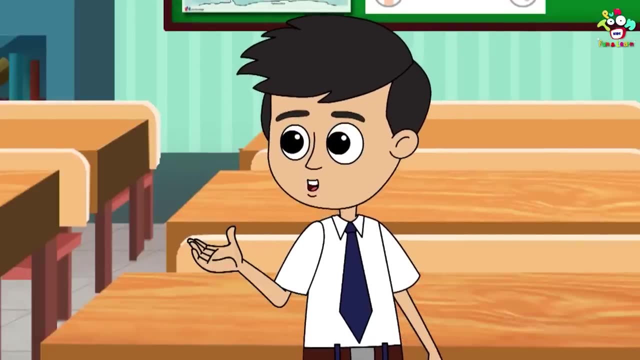 In that way, we need not do any homework at all. Everyone listen If you want to escape from homework and Mishra sir's punishment. tomorrow, for the occasion of teacher's day, everyone bring gifts. Mom, dad, tomorrow is teacher's day. 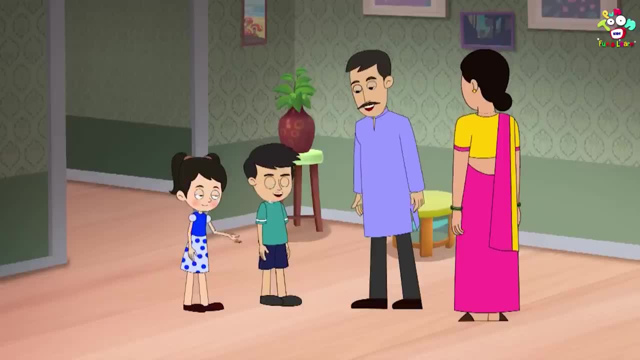 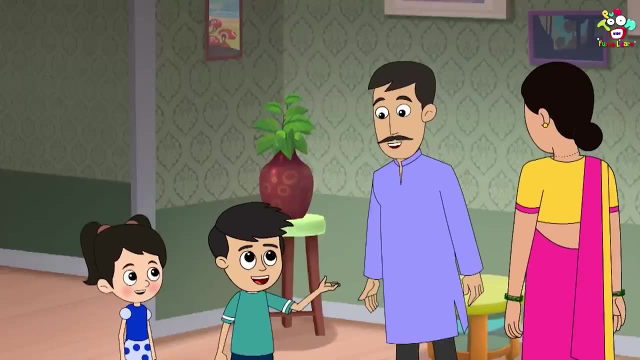 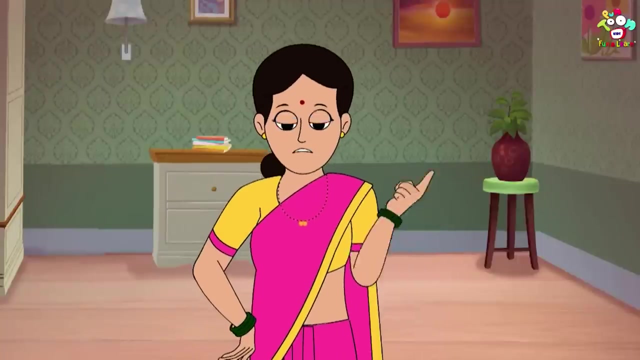 and we want to buy a nice gift for Mishra, sir. Wow, that's a fantastic idea. Now let's go, dad, Let's go and buy a nice gift for Mishra, sir. Yeah, let's go. What go? Don't you see outside it's raining. 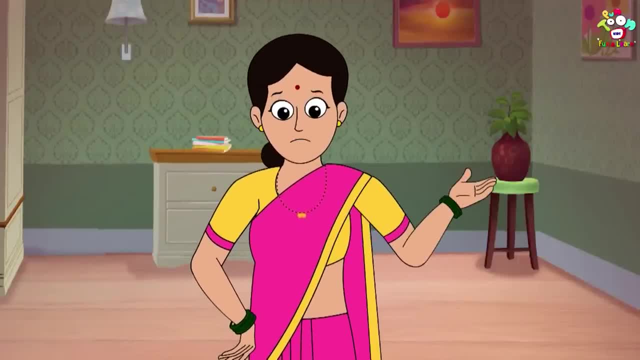 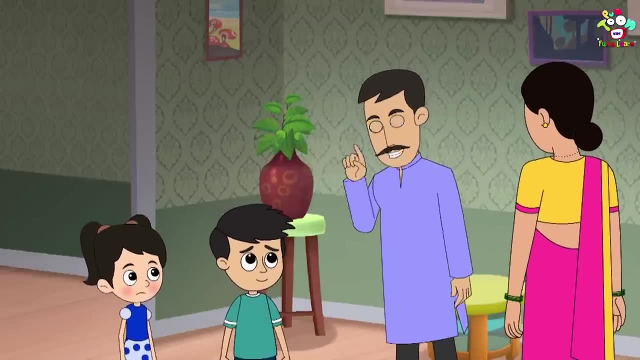 It's raining. cats and dogs- How will we go in such a bad weather? Sorry, kids, It's raining really heavy outside. I'll tell you something: You start doing your homework and as soon as the rain stops, we shall go out to buy the gift. 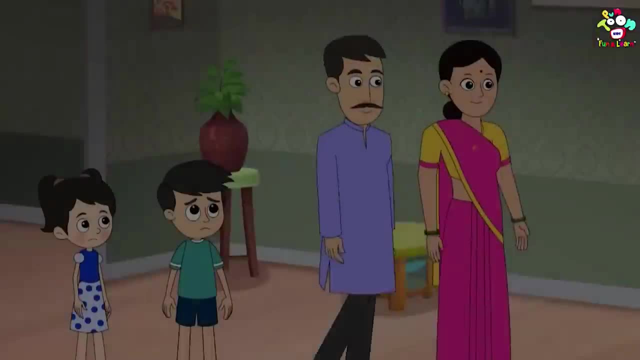 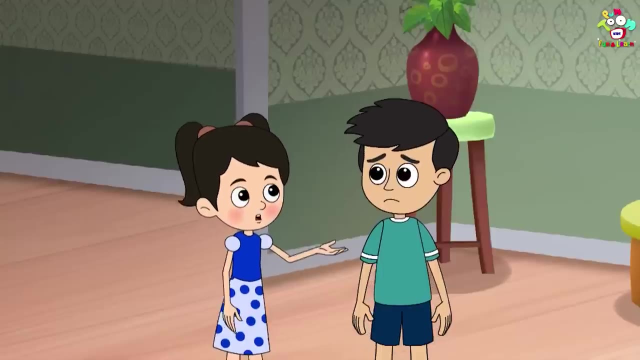 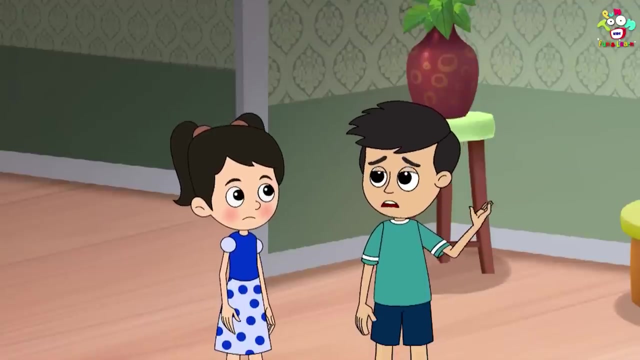 Is that fine, Okay, dad, Dad and mom leaves that place. Now what to do, And what if the rain continues all night? Don't say like that: The rain will definitely stop. Until then, let's try to do some homework. 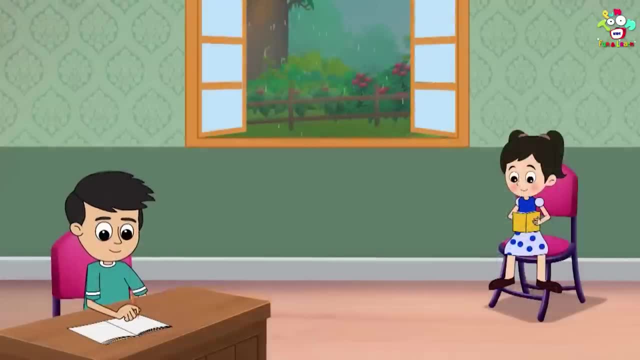 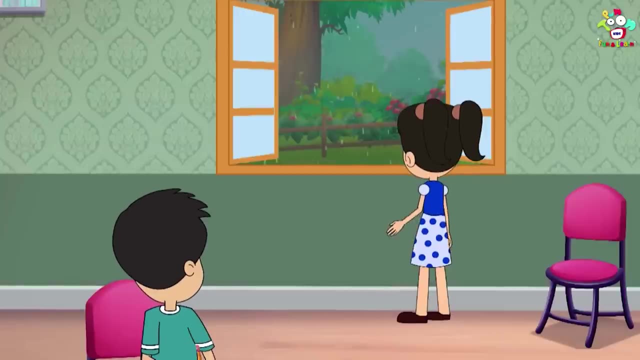 Gattu and Chinky starts doing their homework After a while. Gattu says: Chinky, can you please check whether the rain has stopped or not? Chinky goes to the window and sees that the rain is even harder now. 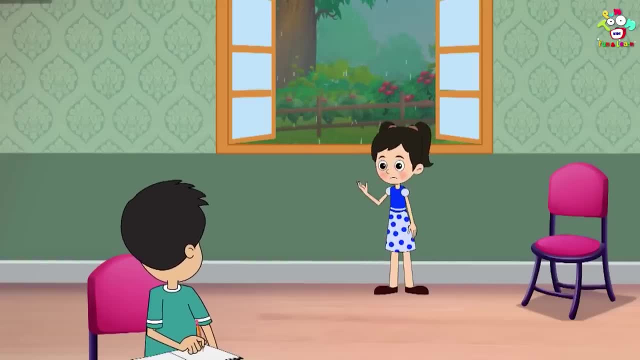 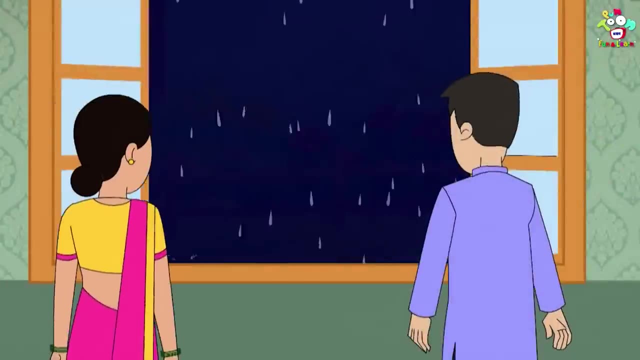 Oh no, it's raining cats and dogs. Okay, then, let's continue to do our homework. Both the kids continue to do their homework. This rain just isn't stopping, And all the shops, too, must have got closed by now. Ask the kids to go and sleep now. 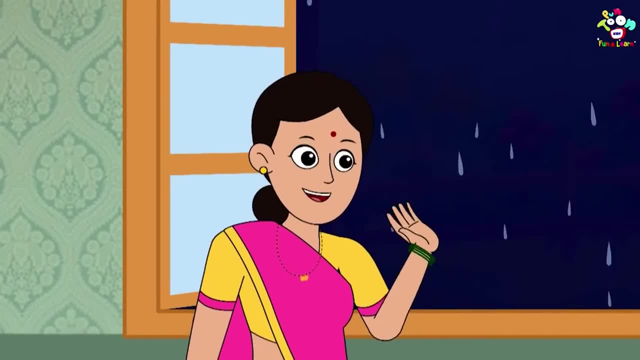 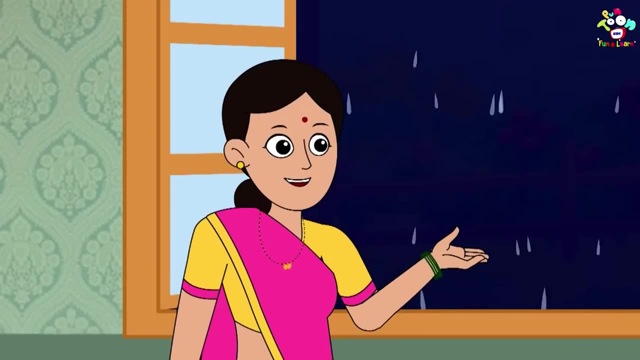 I don't think we can buy the gifts. Leave it After a long time. they both are doing homework. If we tell them they won't do their homework Because of rain, at least homework would finish Well. that's a good idea. 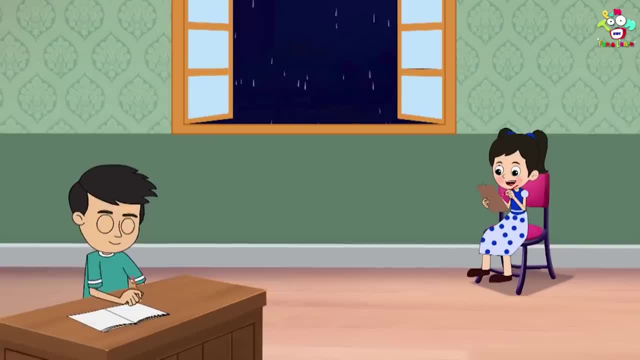 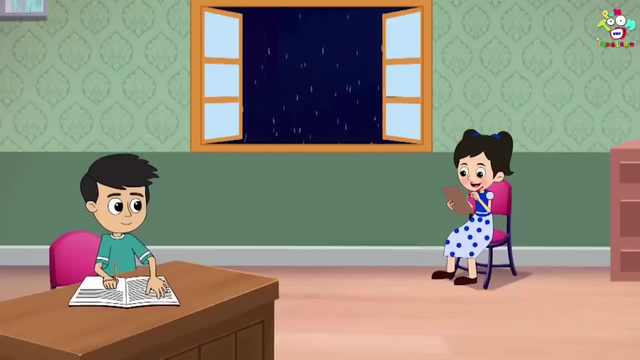 Good night. Dad and mom go to sleep And Gattu and Chinky work all night to finish their homework. They continue to do the homework till morning, 4 am. Chinky has the rain stopped now. at least It hasn't stopped raining. but I am done with my homework. 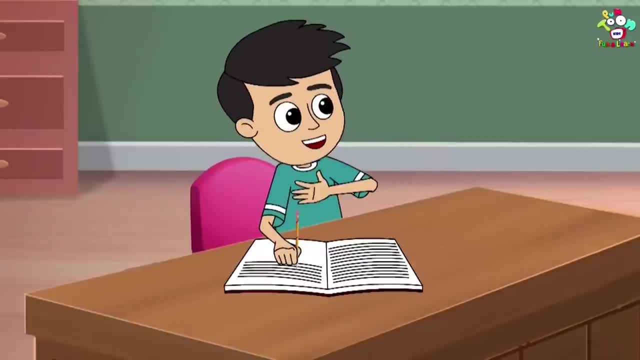 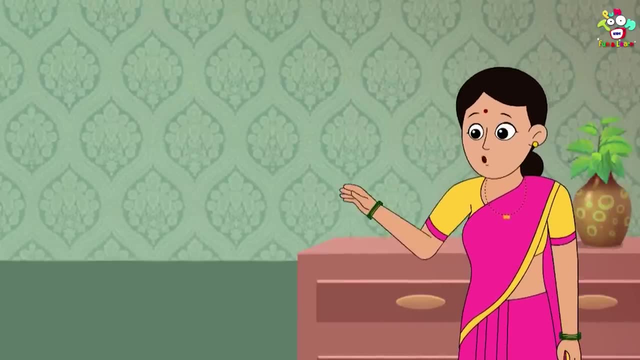 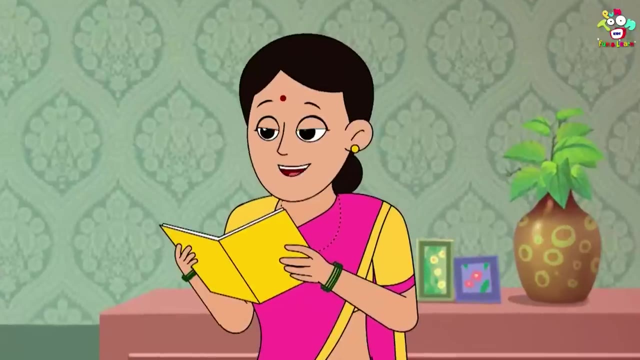 Oh, what are you saying? Even I am left with just one question. That's when mom comes. Kids, it's morning, Sleep. now You need to go to school as well. Mummy, we completed our homework. Wow, we need not buy the gift as well. 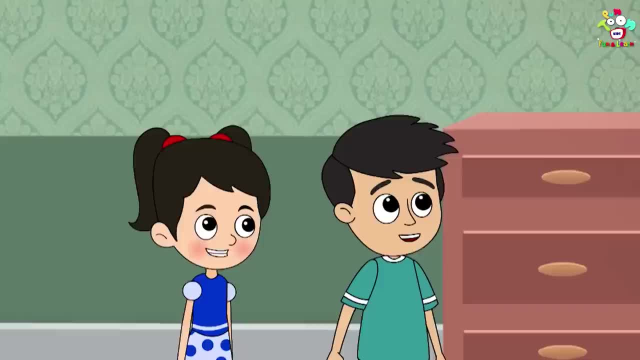 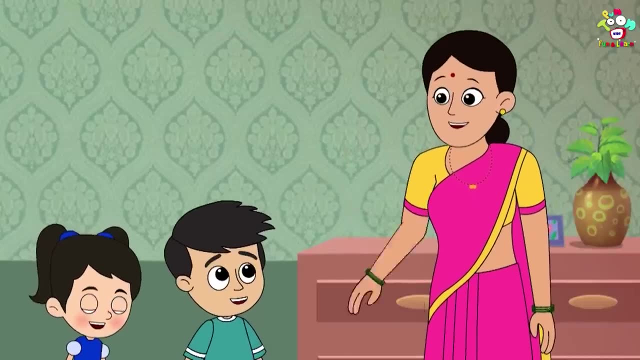 Mishra sir will be happy seeing you. We'll be happy seeing the homework. Oh, yes, we didn't even think about that. Go and sleep now. Mishra sir has got his gift. Mishra sir comes to the class. Good morning sir. 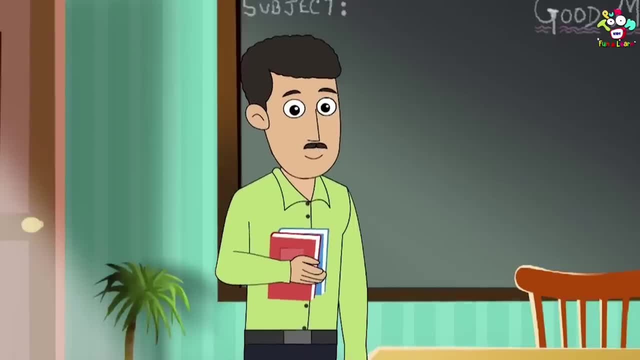 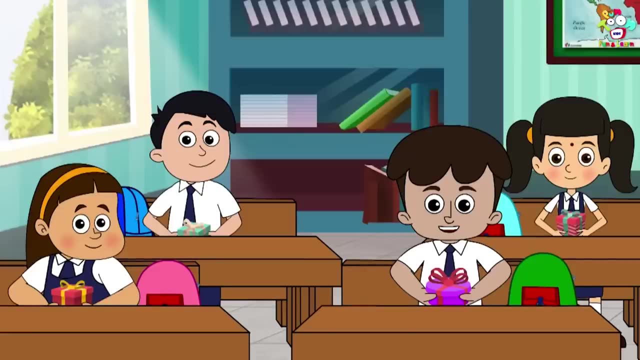 Happy Teacher's Day. Thank you and same to you all. Now come forward and keep all your homeworks on the table. Please do it quickly, As soon as Mishra sir says that all the students get up from their seats and leave their gifts on the table. 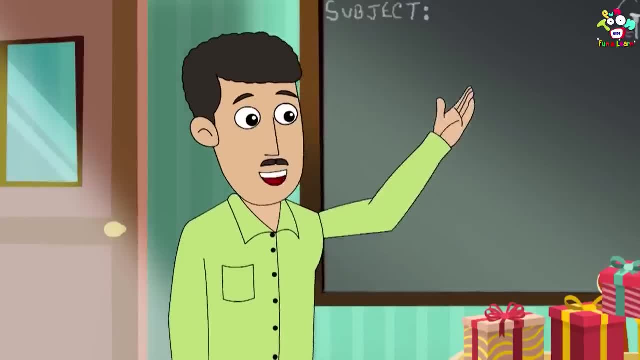 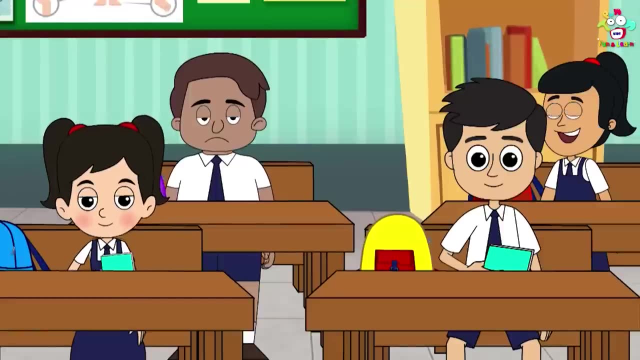 Hahaha, what is this? Instead of notebooks, I have gifts all over the table, No problem at all. Thank you everyone. Gattu and Chinki, where is your gift? Here? we have a special gift for you, sir. 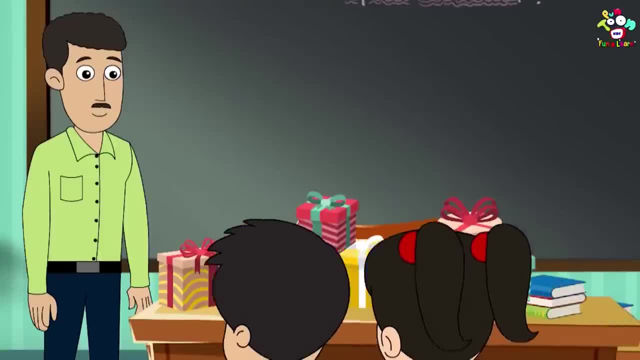 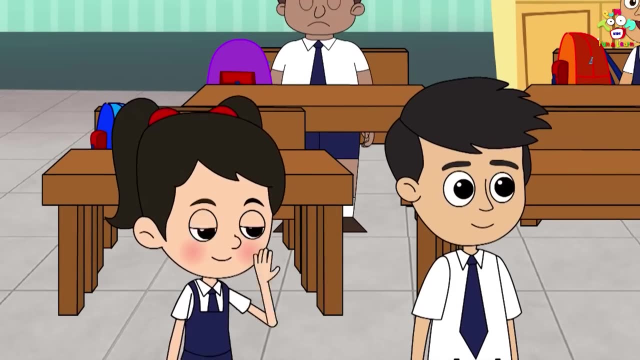 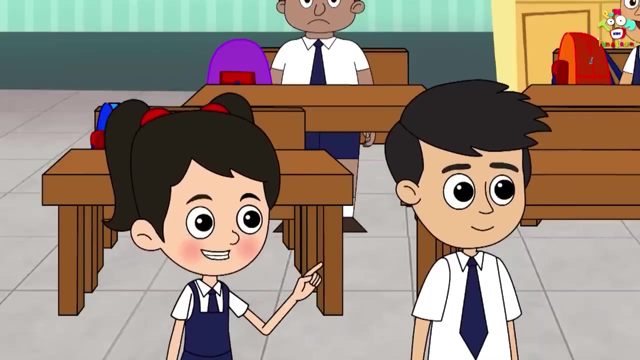 Come on, Chinki Gattu, and Chinki takes their notebook and shows it to Mishra. sir, Here is your gift. We sat the whole night and completed all the homework which you gave. There is nothing left now. Please do check if you want. 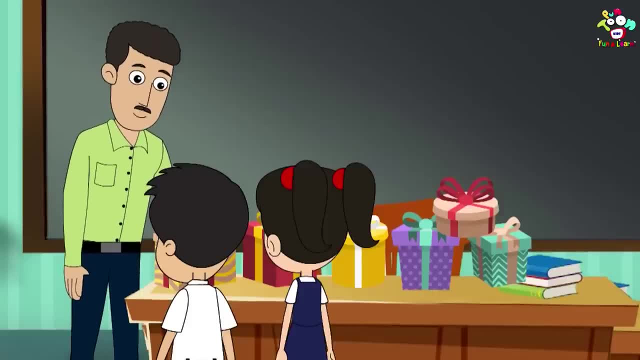 What? Let me see. Mishra sir opens the notebooks and starts to check them. He gets shocked to see that Gattu and Chinki have finished all their homework. Wow, Gattu and Chinki. well done, Kids. today is Teacher's Day. 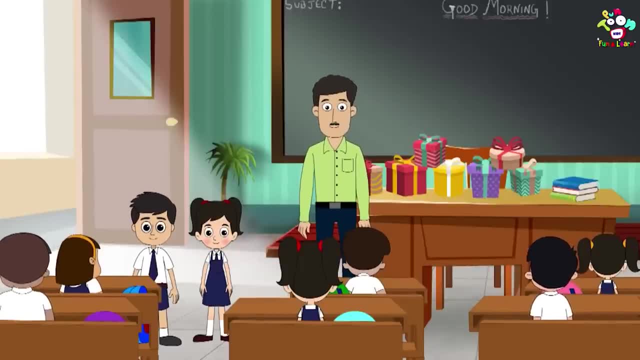 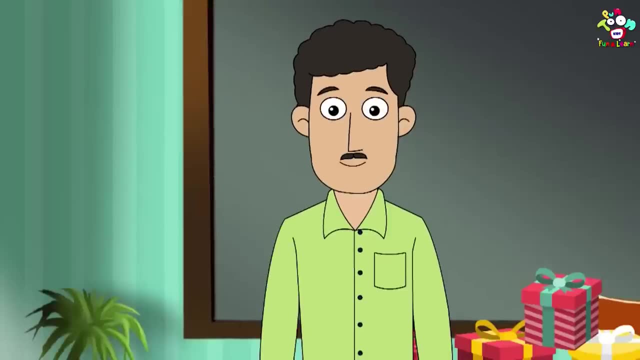 You all have given me lots of gifts. I liked it a lot. This gift of Gattu and Chinki is what I like the most. Kids teachers always think good for you. You become clever and grow well in your life. That's what teachers wish for. 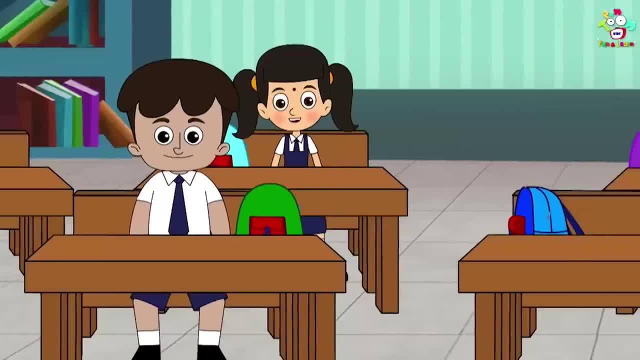 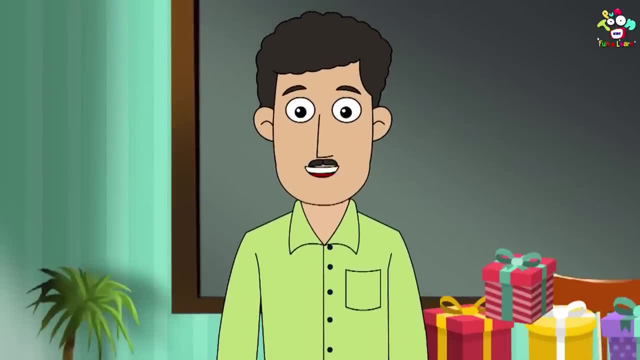 Kids should listen to their teachers, Stop always making noise in the class and do their homework, And if this is how the class would be, teacher's wishes are fulfilled. If you all also understood the same, I'd be the happiest person. Don't worry, sir. 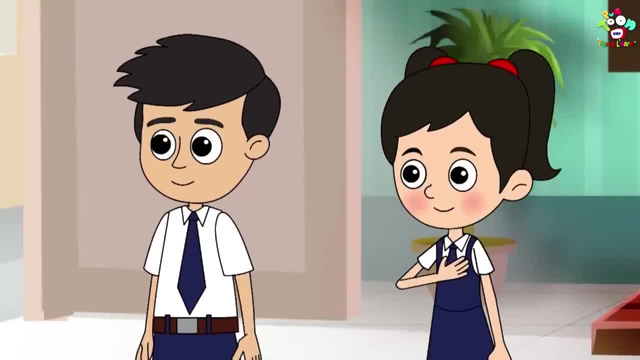 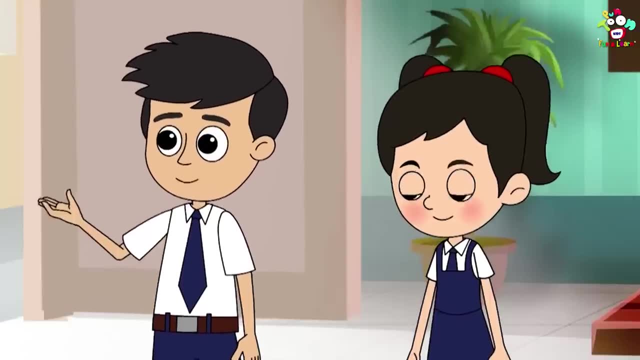 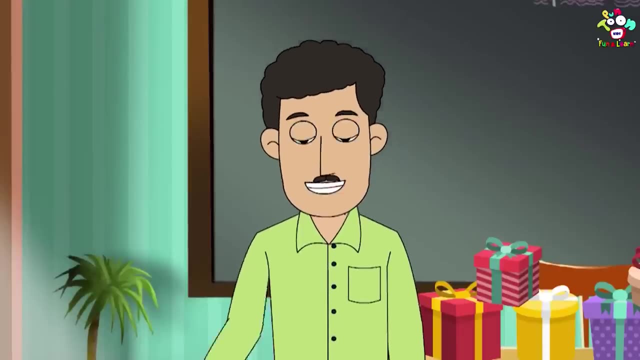 From now on, we will do whatever you say, Sir. we have completed our homework. Now we are going to help others to complete their homework. That's a great idea. Now, that is what I call Teacher's Day: real celebration.